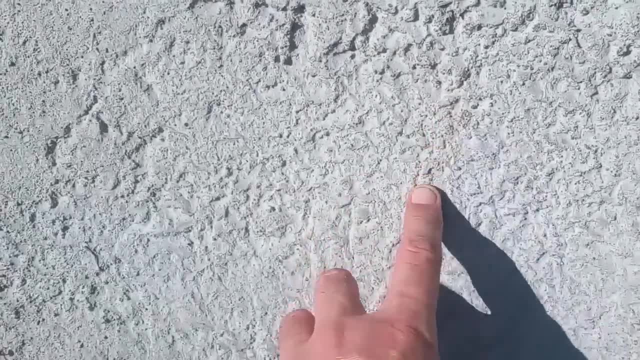 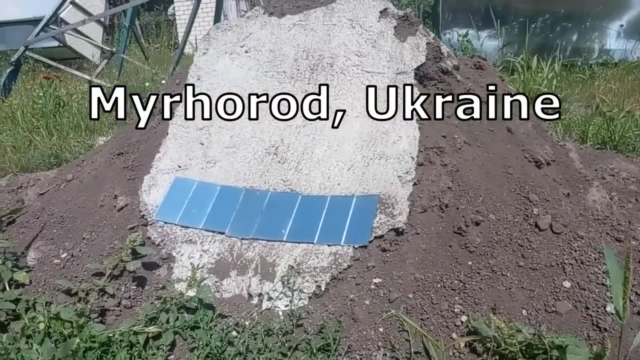 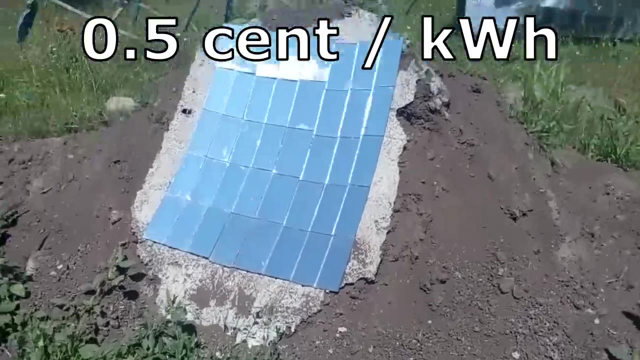 I remind you that my goal is not entertainment. My goal is to find the best method of converting solar radiation into thermal energy at the lowest cost. My goal is to produce solar thermal energy with temperatures up to 400 degrees Celsius at a cost of half a cent per kilowatt hour, and it is about 10 times cheaper than the cost of heat from natural gas. 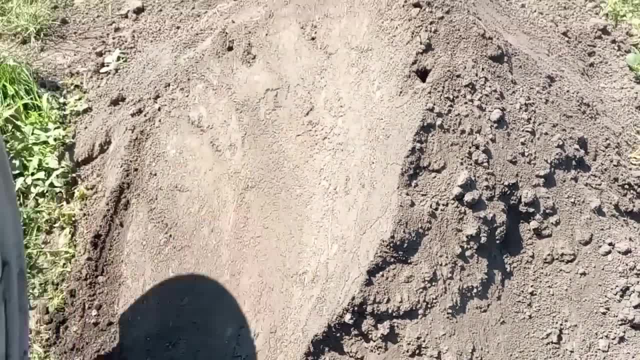 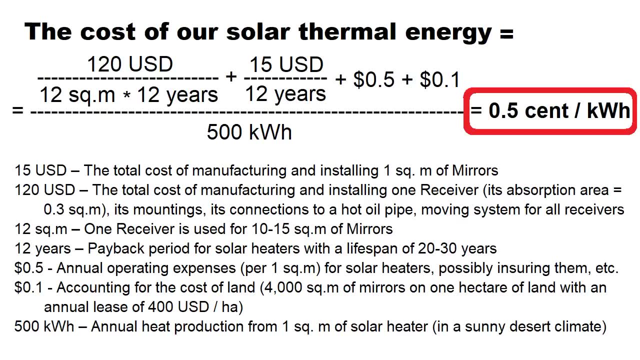 Why we should get rid of this metal plate is explained by this formula Here. it requires that cost of solar thermal energy- half a cent per kilowatt hour, which is needed to produce very cheap solar electricity that is cheaper than electricity from thermal and nuclear power plants. 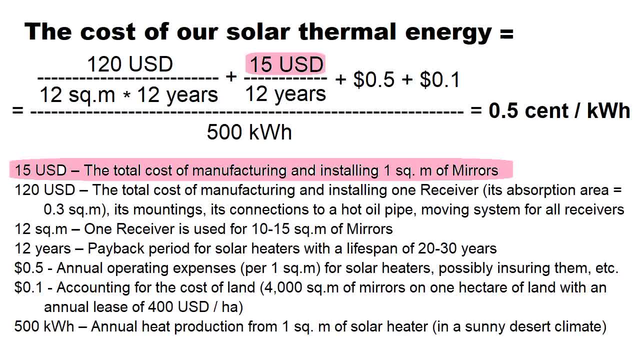 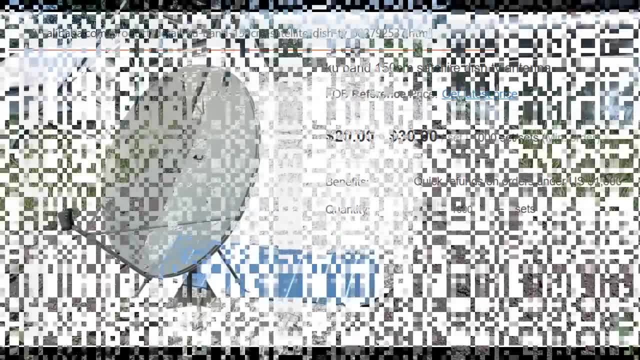 Here we see that the total cost of our mirrors should be $15 per square meter, which is approximately equal to the cost of a metal plate. But we also have to spend money on the glass mirrors, wages for workers, building an earthen berm and other expenses. 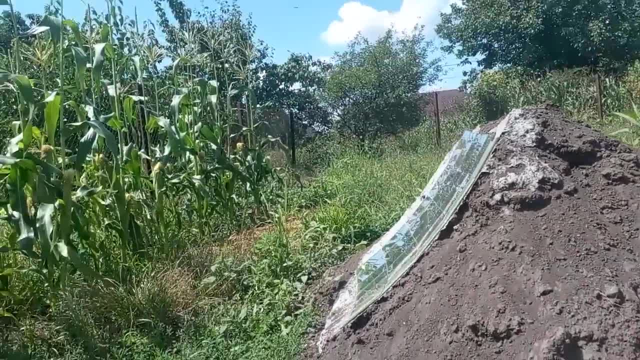 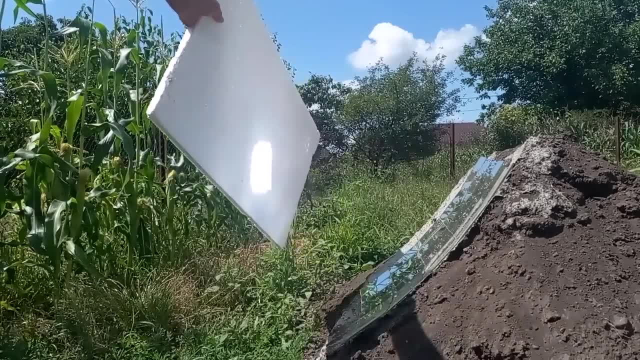 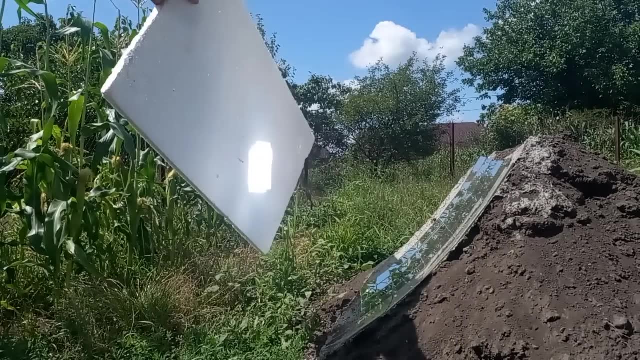 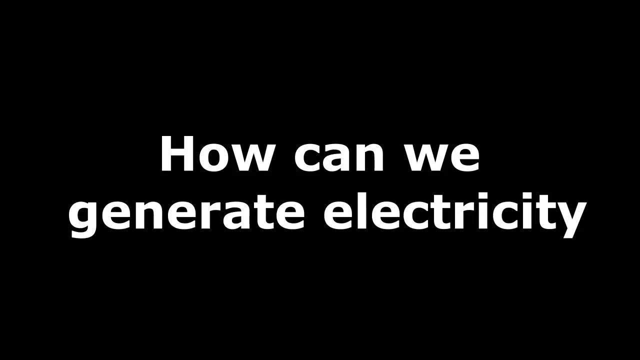 However, let's look at how my cheap mirror dish focuses solar radiation. Here we see spots of solar radiation from each of my small mirrors. We also see that the spots of all mirrors are trying to unite at this point, and now I will describe how this solar energy can be turned into cheap electricity. 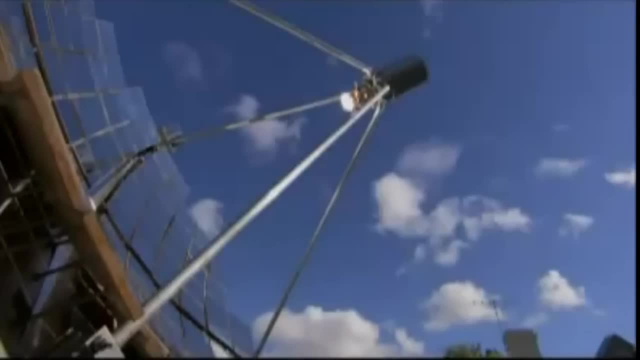 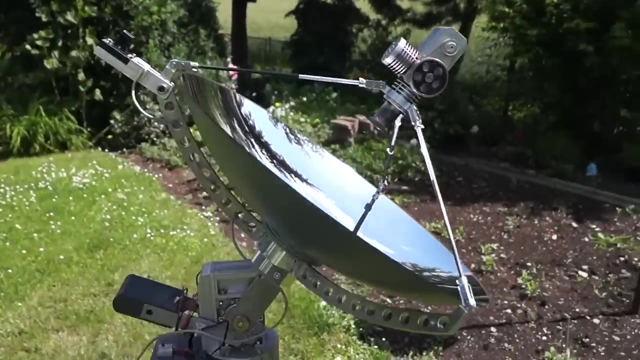 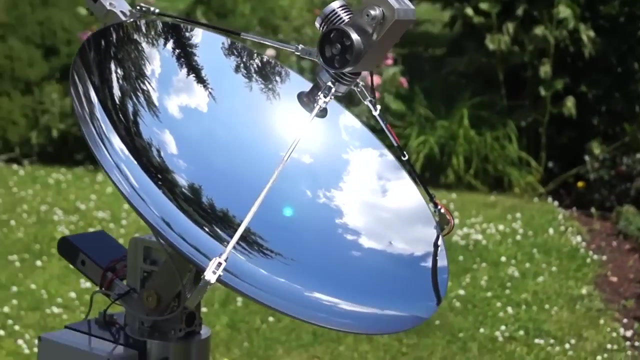 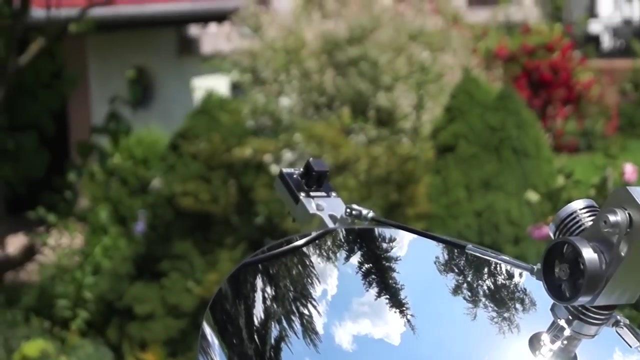 Now I am showing the first option, where a small solar panel is located here. This is the second option, which suggests that a stilling engine be located here and it converts the thermal energy into rotation of an electric generator. Unfortunately, these two options are not suitable for us because they only produce electricity during the sun, similar to these well-known solar panels. 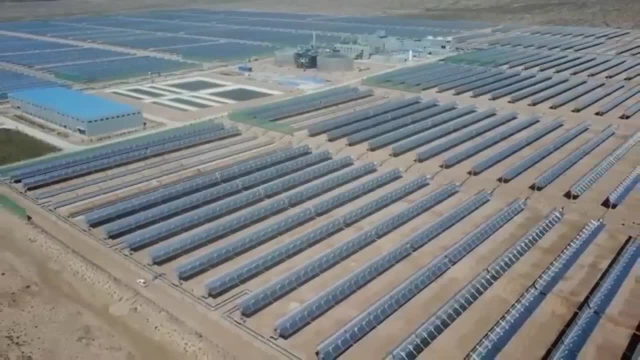 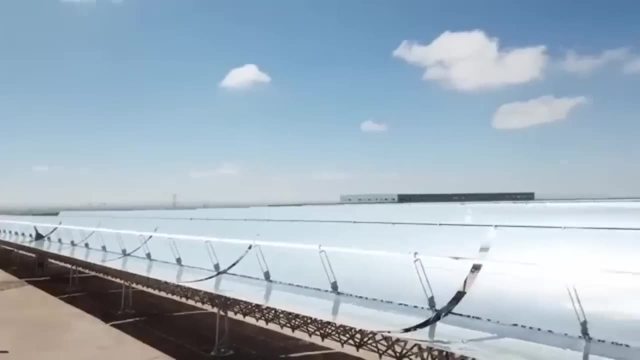 At the same time, we need a solar power plant that will give us electricity 24 hours a day. Electricity both day and night can be produced by our third option, which is used by solar power plants of this type, and now I will quickly remind you how they work. 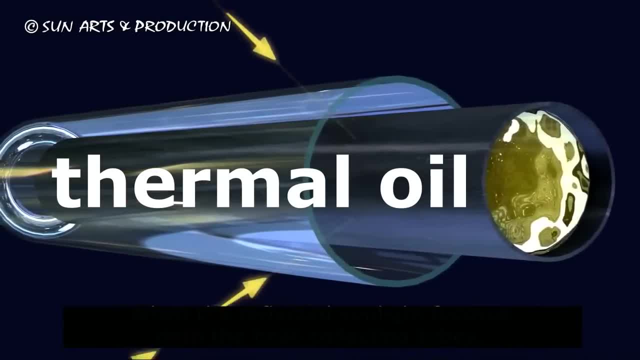 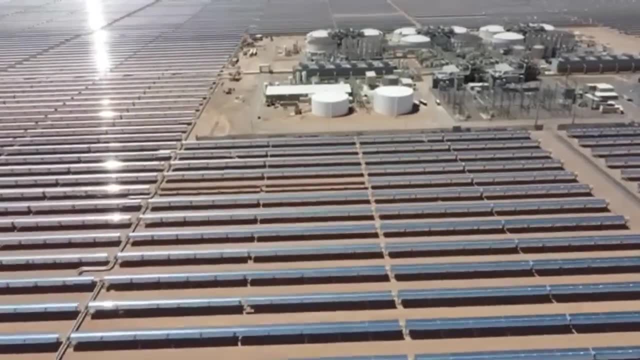 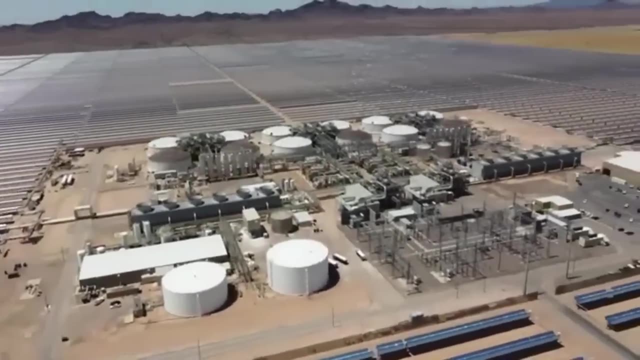 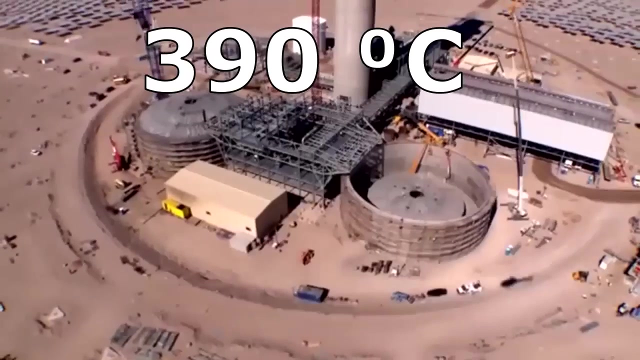 When the sun appears, its radiation heats thermal oil inside these receivers to temperatures of almost 400 degrees. This hot oil moves to the center of the solar plant where its proportion produces steam for a turbine which generates electricity. The rest of the oil comes to such heat storages, where the oil heats huge masses of substance to a temperature of almost 400 degrees. 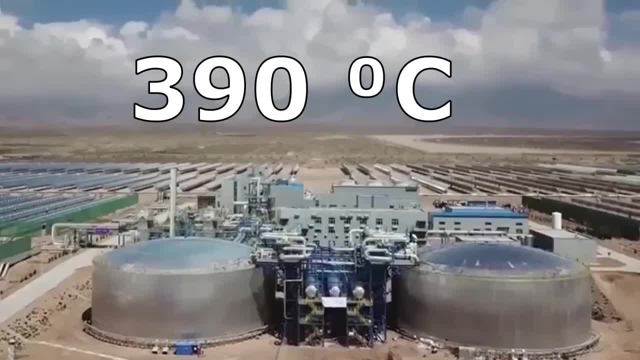 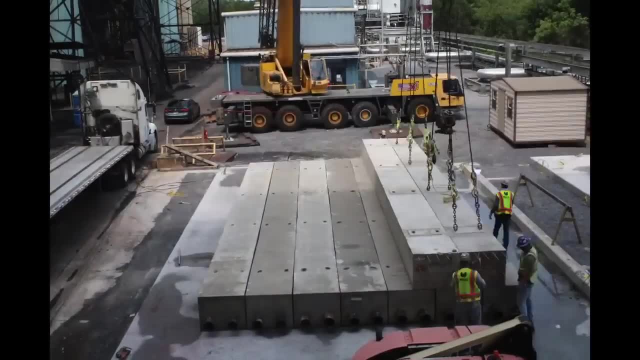 A few hours later in the evening or at night, that hot substance of the heat storages will produce steam for the same turbine. An old video 9 months ago described various types of heat storages where that hot substance is concrete, sand or other cheap substances. 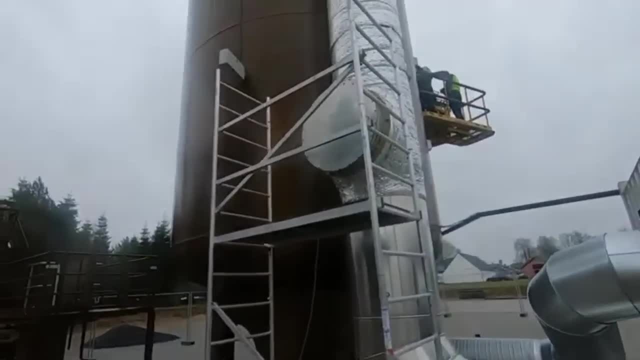 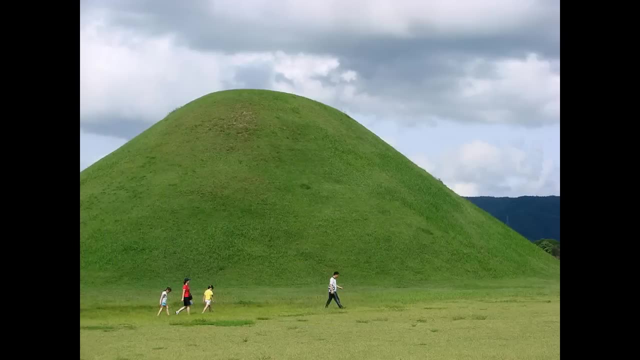 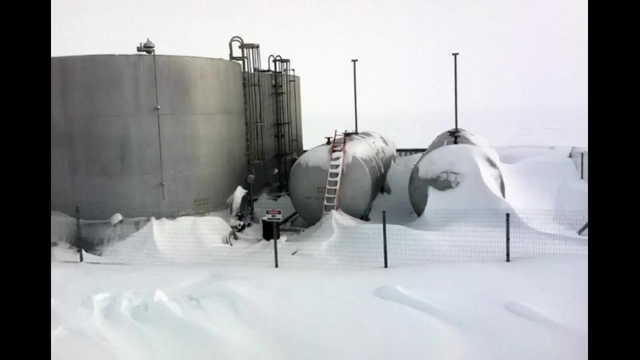 Heating these substances to several hundred degrees allows the storages of thermal energy to generate electricity for several non-solid days in a row. Moreover, a very large heat storage can store thermal energy for several months to transfer the energy from summer to winter, which was described in this old video of heat storage. 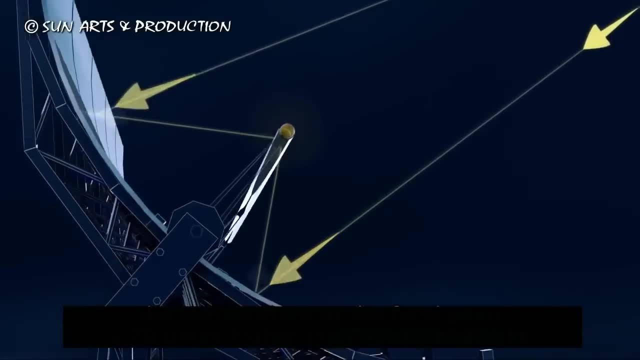 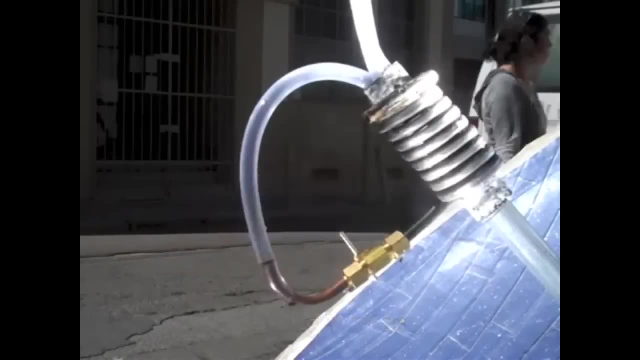 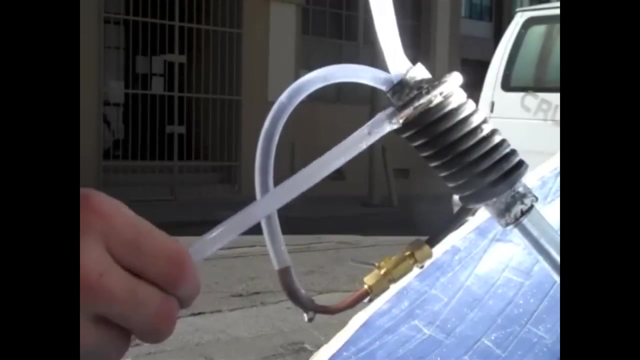 So we understand that our mirror dish must also have a relative of this receiver. and now I am showing an example of the receiver we need from another blogger. This receiver heats water for hot water supply, but we understand that it can be heating that thermal oil a few hundred degrees. 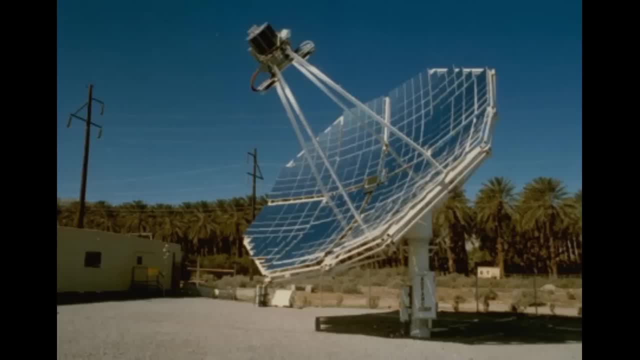 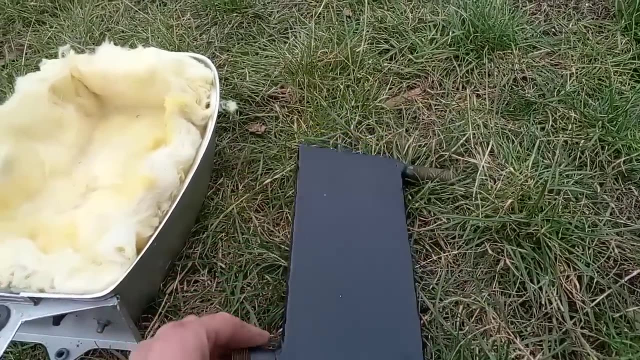 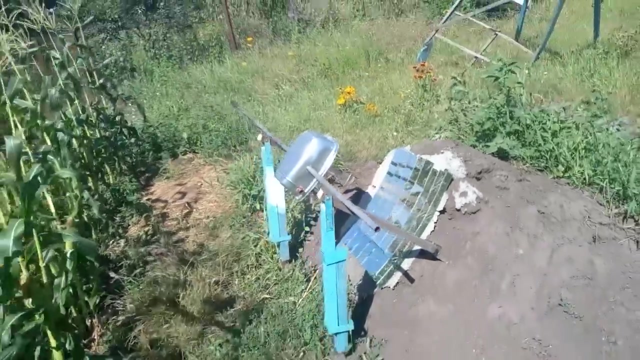 or it can be these examples- with a heating temperature of about a thousand degrees Celsius. This is an example receiver for my mirror dish and previous videos have shown how it works, But this receiver must be several tens of times less than the total area of the mirrors. 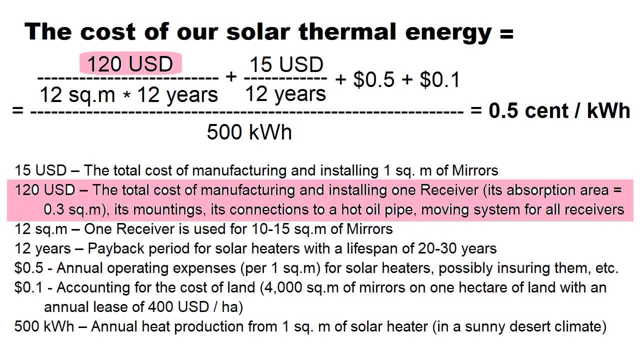 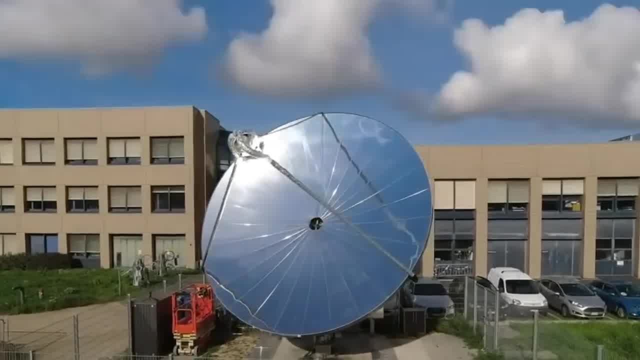 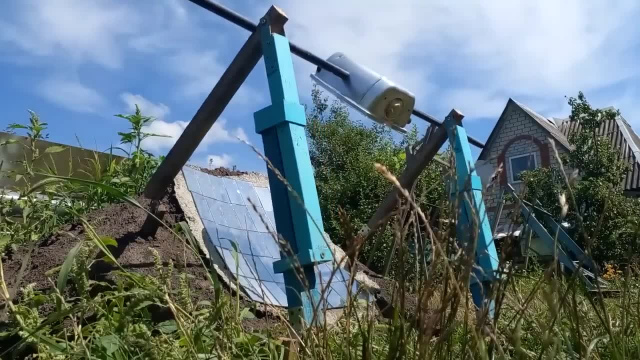 otherwise its cost will be higher than these requirements. Now I remind you that usually mirror dishes should constantly move according to the movement of the sun across the sky, But I propose to replace this movement of the dishes with such a movement of receivers, and how it works will be shown by the following experiment, where this mirror dish is replaced by this concave mirror. 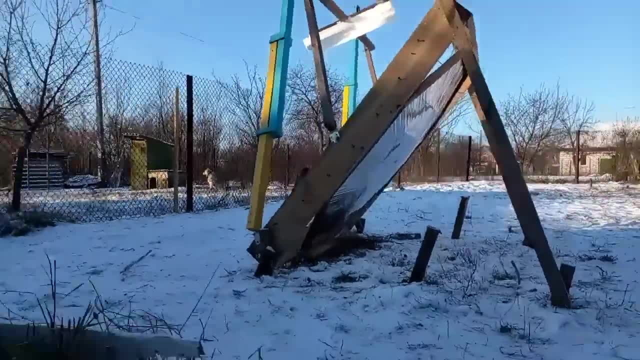 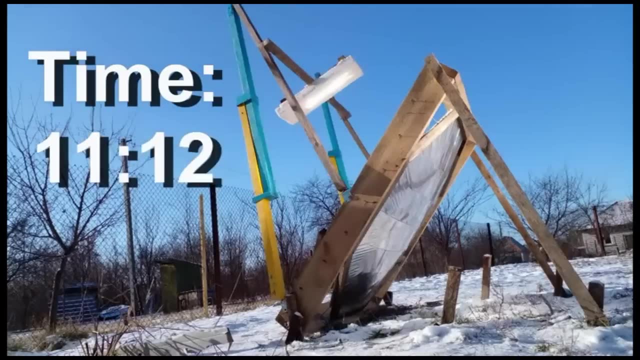 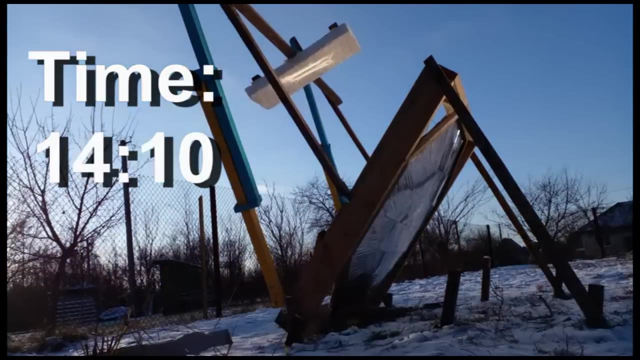 The west-east line is here and we see solar radiation from the concave mirror here. These are points in time of one day from morning to evening. We see that this part of solar radiation from the concave mirror is constantly inside this white screen that is used instead of our receiver. 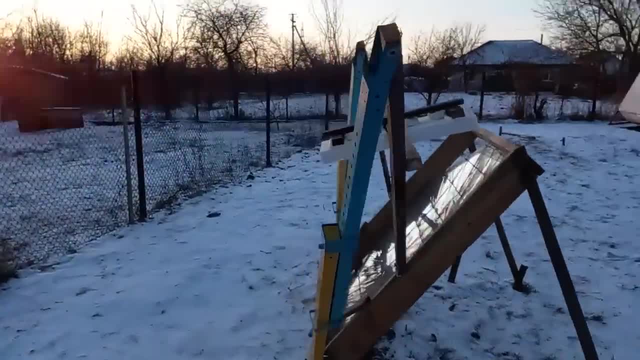 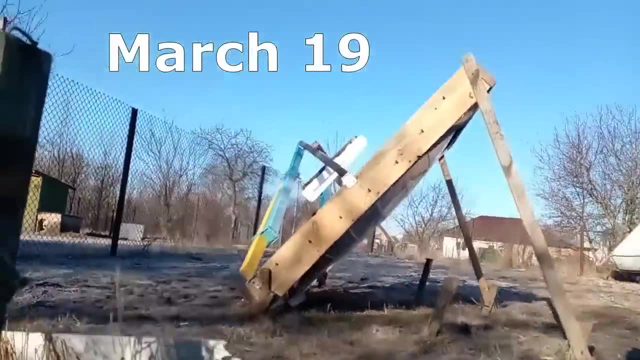 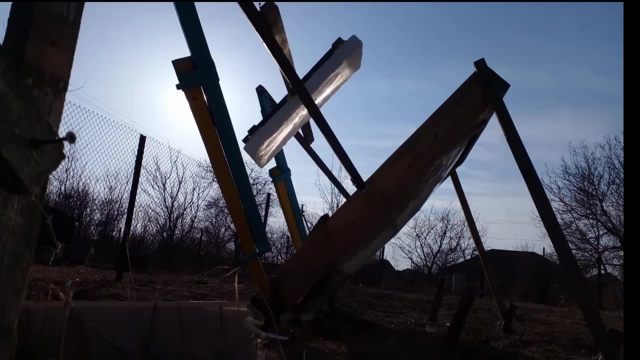 which moves according to the movement of the sun across the sky. This was the case around the winter solstice, but now I will show the same experiment, but around the spring equinox. We see that this part of solar radiation is also inside the white screen all day long. 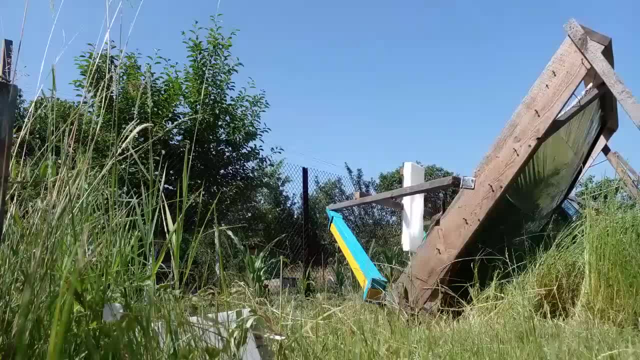 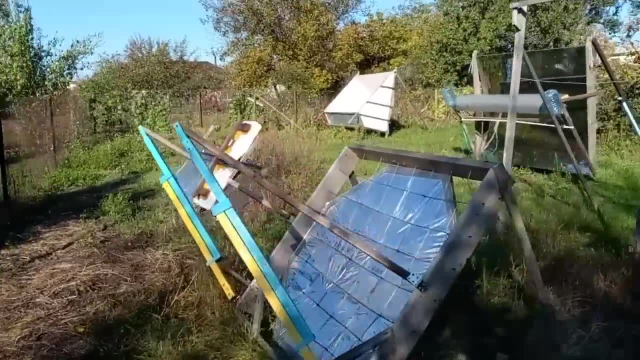 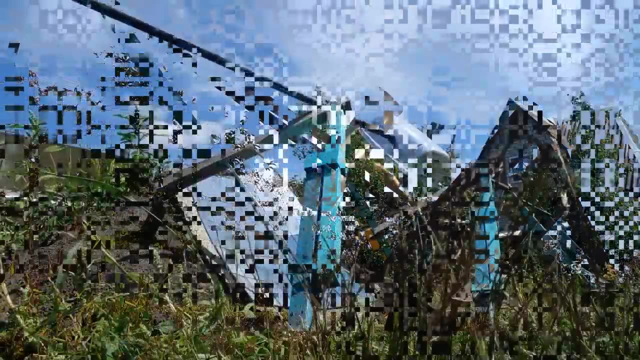 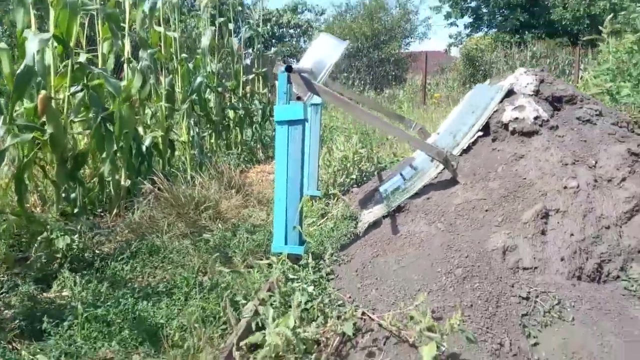 This is the same experiment, but around the summer solstice, and we can notice that this part is also constantly inside the white screen. This is the fourth k-period around the autumn equinox. In addition to these movements from morning to evening, we also have to make the following changes in the position of the receiver, about 12 times a year. 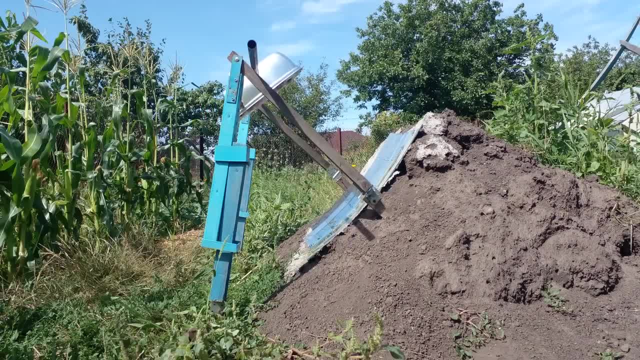 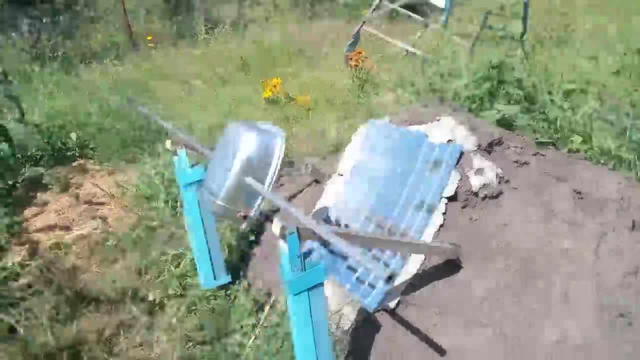 This is the position in June, and then we take these six steps and reach this position in December, and after that we take six steps in the opposite direction until the summer solstice. Here we see devices for those changes in the position of the receiver. 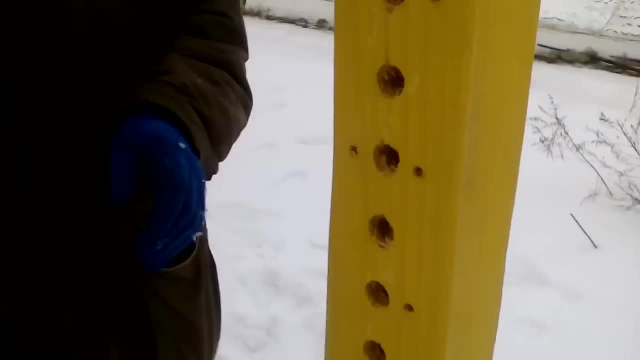 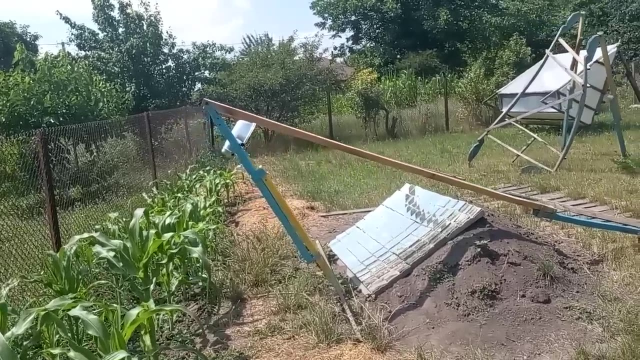 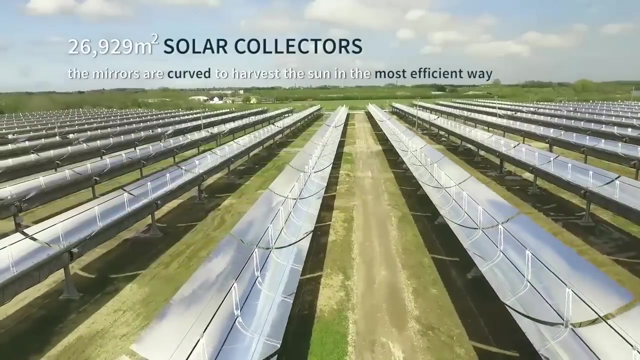 and now I am showing how I do similar actions on my solar station. I also remind you that my previous video described a different option for mounting the receiver, and also this option. It is obvious that our mirrors must form such long rows according to the rules which are shown by me in this primitive example. 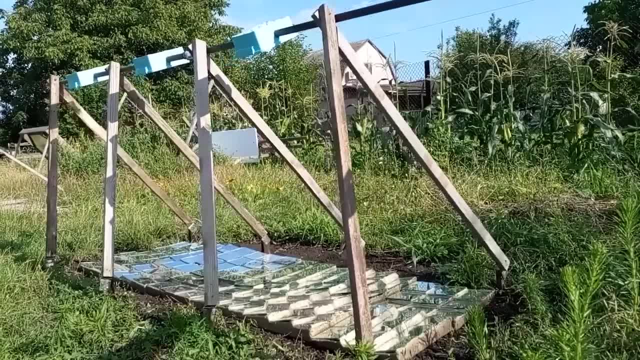 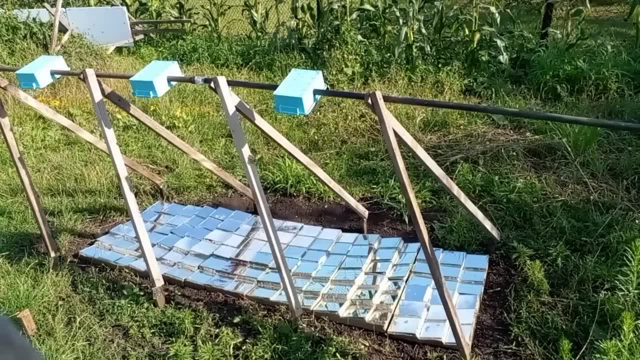 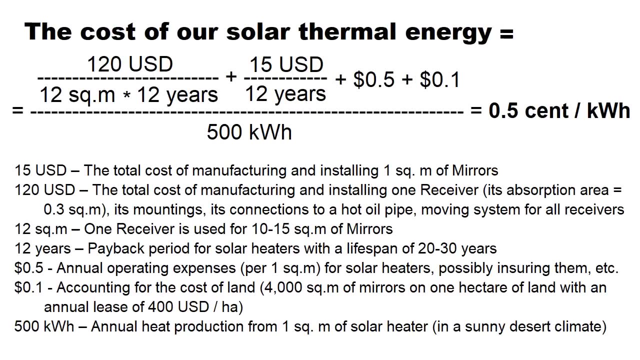 Here we see several receivers of one short row and, for example, this receiver is the focus point of the solar radiation of these mirrors, but it is obvious that there must be several hundred mirrors here. In addition, these widths should be several meters, because small mirror dishes will worsen these targets. 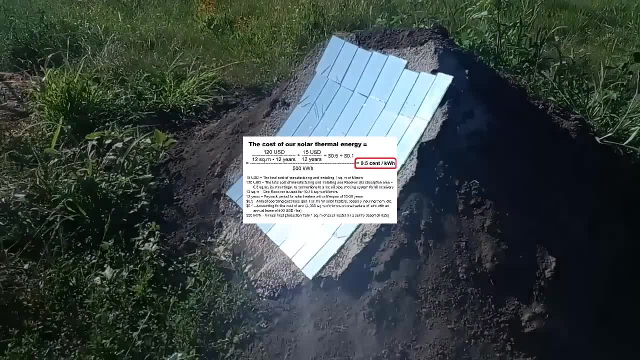 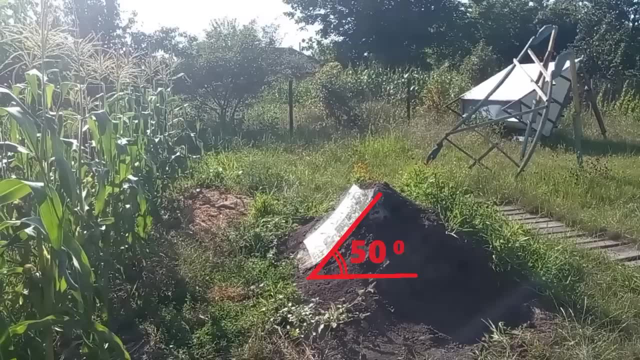 which leads to a noticeable increase in the cost of our energy. We can notice that our mirror dish must be placed on the surface of the earthen berm, and this angle is 50 degrees because it is equal to the northern latitude of the place where I am. 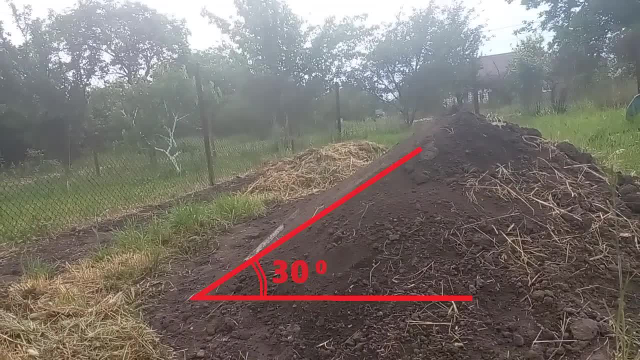 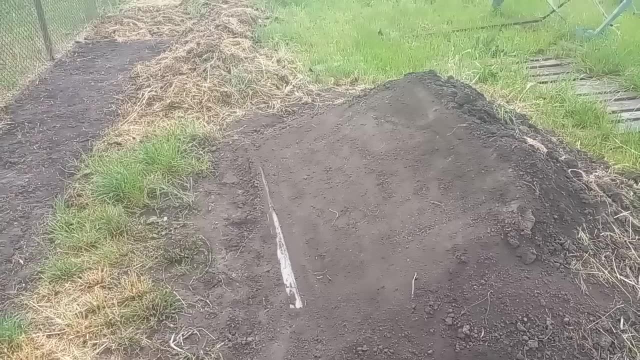 This is a berm for most southern countries at 30 degrees north latitude, and it is obvious that countries near the equator do not require any berm when the concavities for our mirrors can be made on the natural surface of the earth.